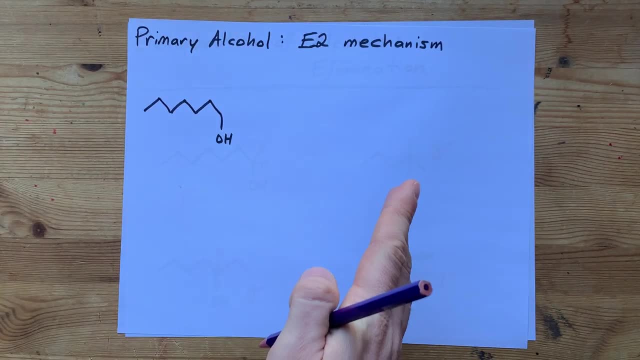 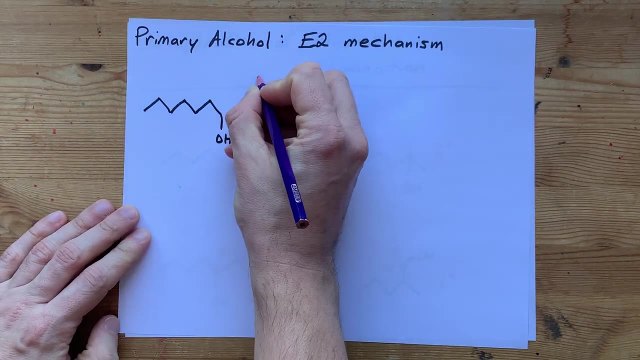 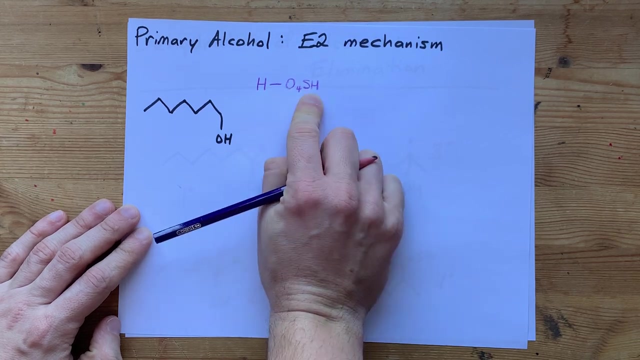 two things colliding in the rate-limiting step. The rate-limiting step, I believe, is the second one here, so let's just talk about what's happening here first. The very first step of this is for some acid. I'm going to use H2SO4 here and I'm going to 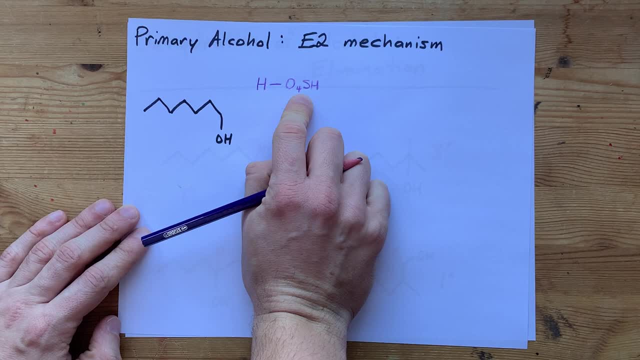 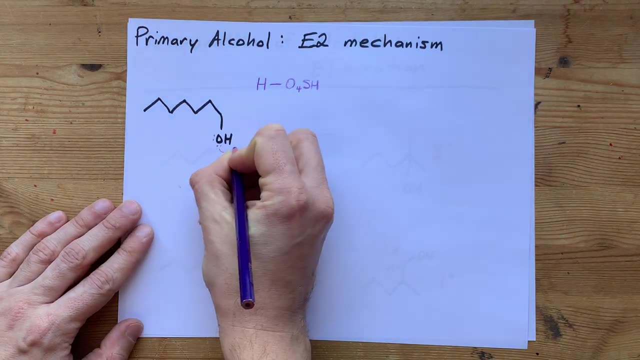 draw it in a weird way. I just want to emphasize that the H isn't connected to anything other than the other oxygen here, and the lone pair on the OH will take the H2SO4 and the H2SO4, and the lone pair on the OH will take the H2SO4 and the H2SO4,. 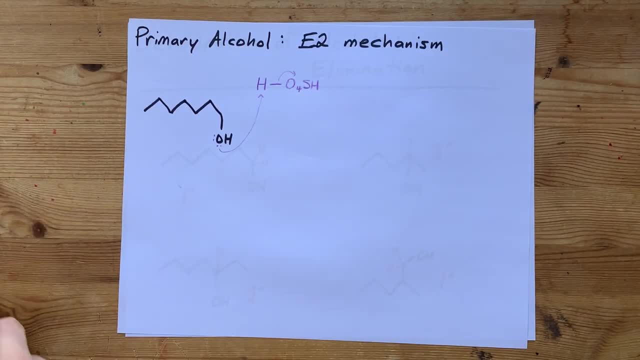 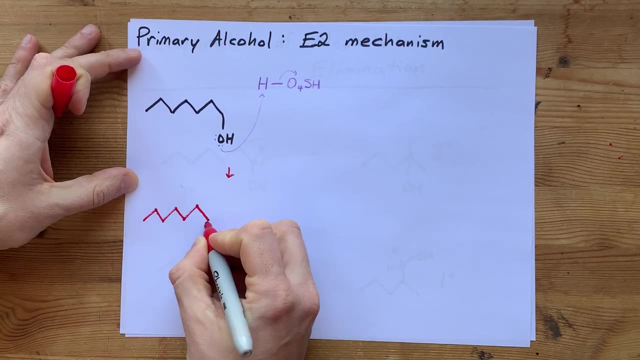 and the lone pair on the OH will take the H2SO4 and the H2SO4, and the lone pair on the OH will take that hydrogen away and leave a minus charge on the anion. The products we get out of that are the same long carbon chain we start with. 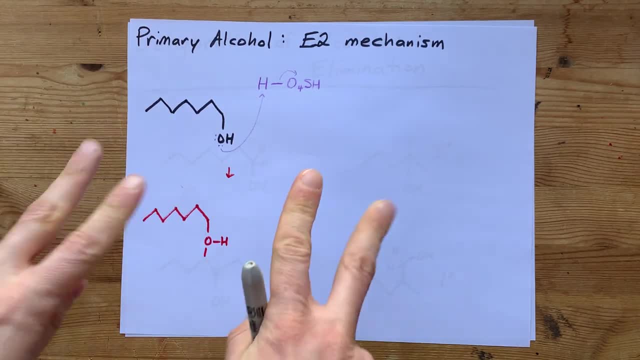 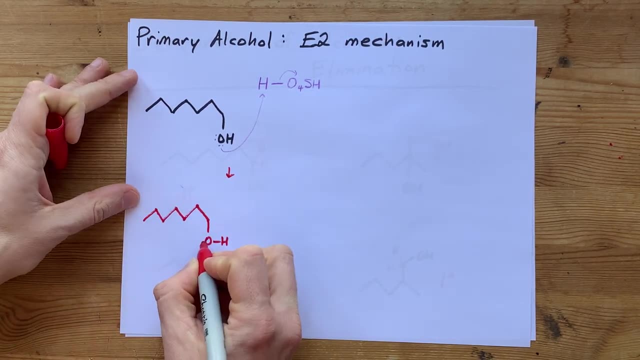 but now, instead of it being an OH group, we have what's called an alkoxonium alko-oxonium ion. It's basically a carbon chain where the OH has been converted to an H2O and there's still a. 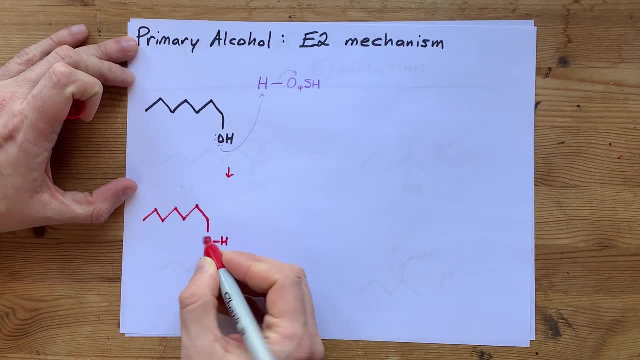 covalent bond between the oxygen and the carbon, but because water is such a great liquid, it's not going to be able to convert the oxygen to an H2O, So leaving group. it's a severely weakened bond and it's very open to being broken. 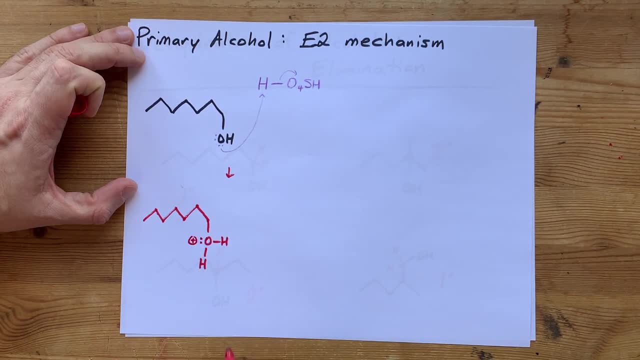 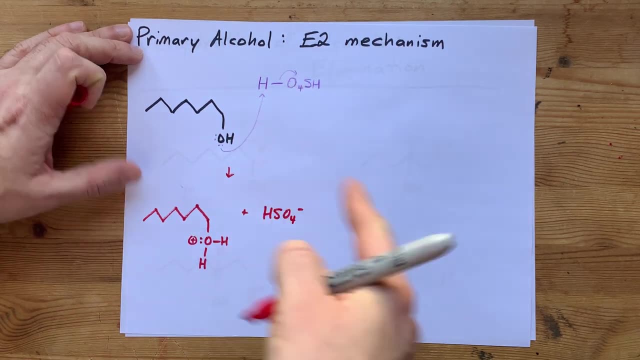 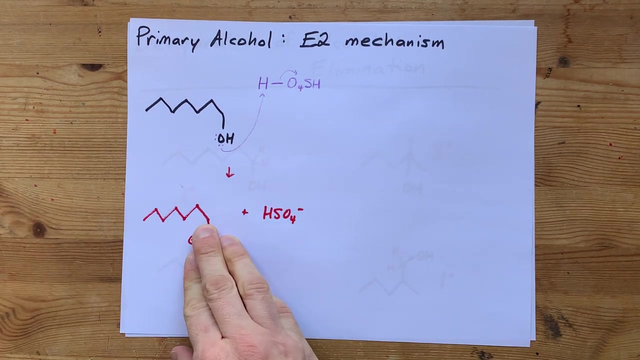 We still have one lone pair on the oxygen and a formal charge of plus one That's countered by the extra minus charge left on whatever the conjugate base of the acid you used was. Now the question is if we're going to eliminate this part of the molecule. 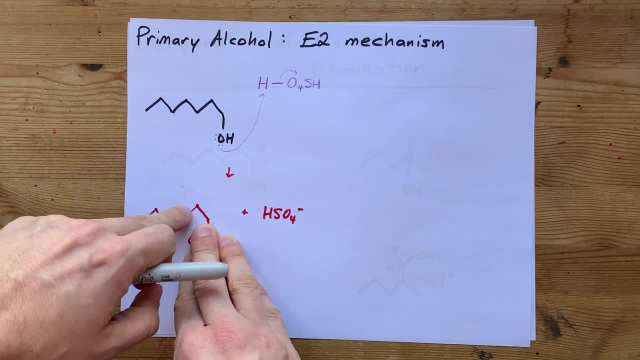 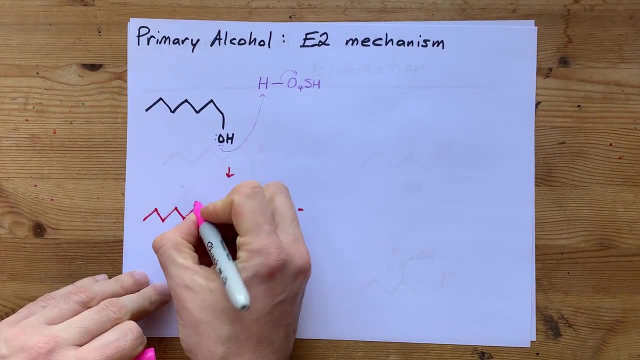 we need to eliminate a hydrogen off of the next carbon in order to leave, believe me, the H2O. So if we're going to eliminate this part of the molecule behind the double bond, I'm going to draw in those hydrogens here. That next carbon here has. 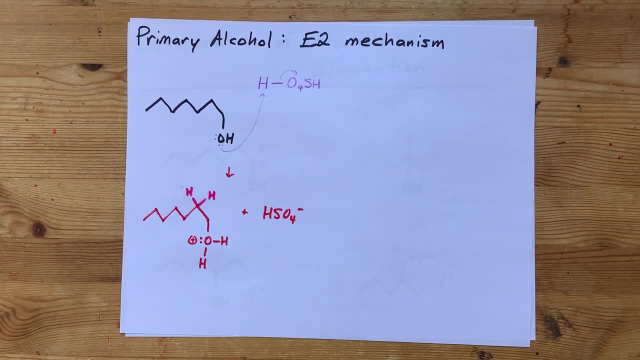 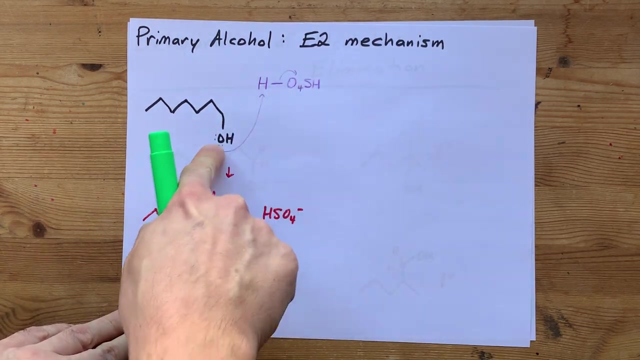 one, two extra hydrogens on it. Now, technically this one does as well, but I didn't need to show those. What's going to happen here is the conjugate base of the acid, which, again the acid gave away its H to make the OH into OH2, is going to steal. 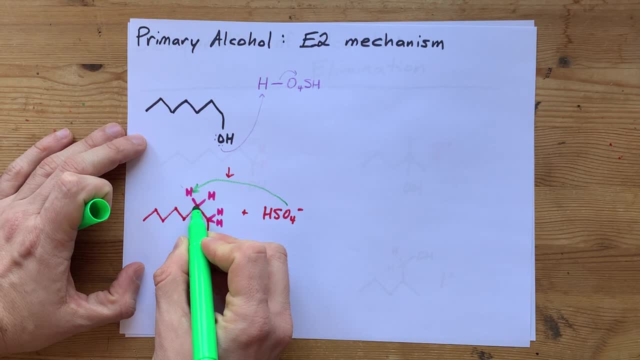 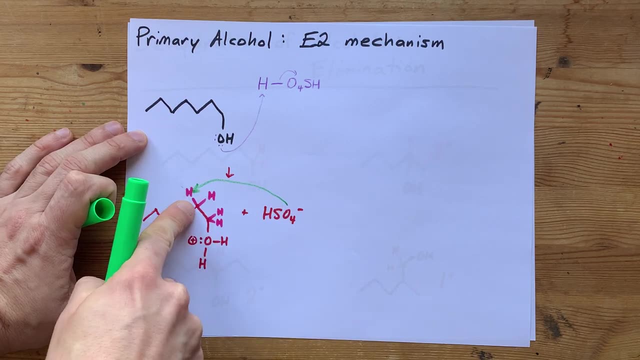 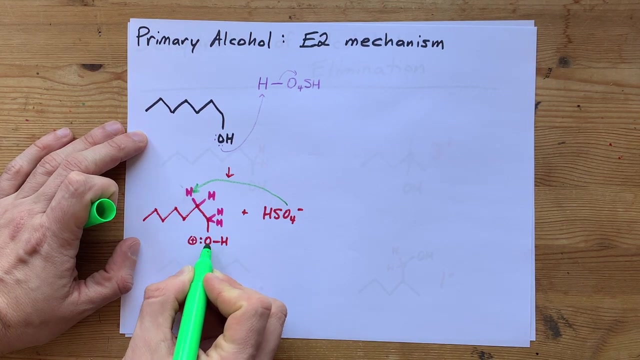 one of the hydrogens on the carbon next to the carbon that has the OH on it. It's stealing the H and those electrons have they need to go somewhere. They're attracted to this bond because the electronegative oxygen is sucking electron density in this direction. So 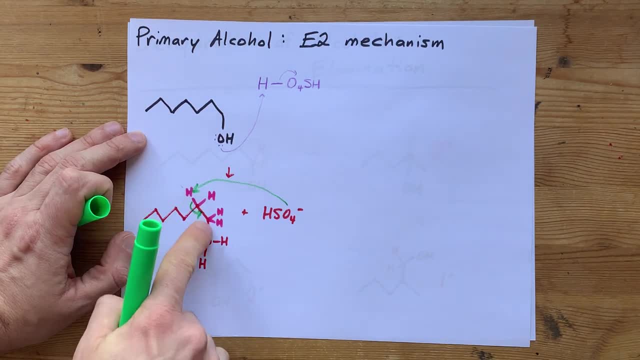 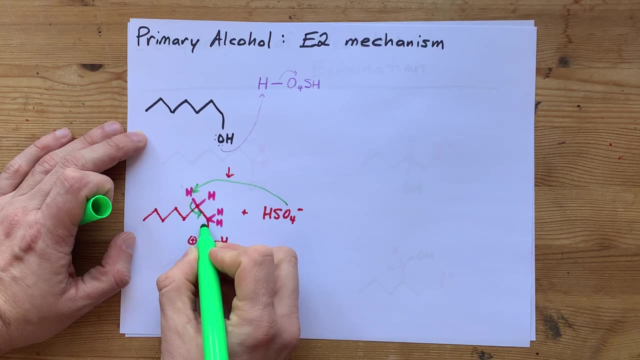 those electrons end up going into or between those two carbon atoms. but each carbon can't have more than four. So if we're going to eliminate this part of the molecule, we need to eliminate this bond. So this covalent bond breaks and those electrons are not absorbed, but they're taken by. 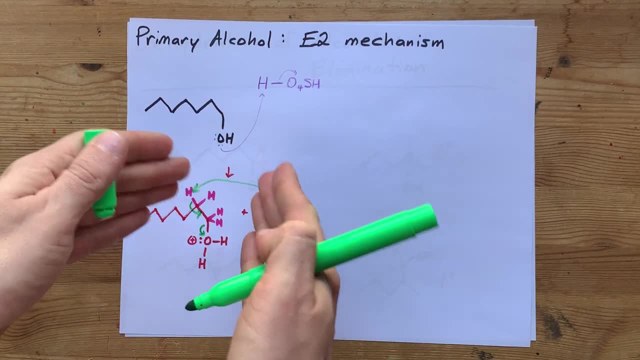 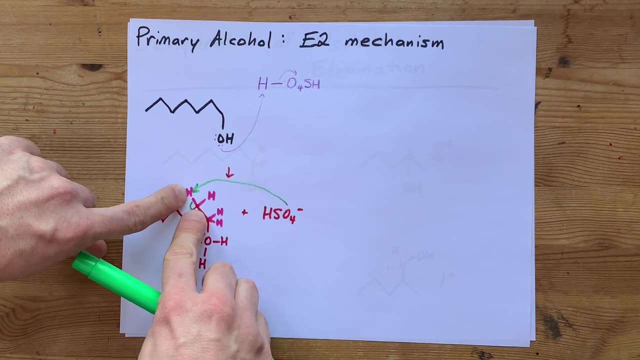 the oxygen. because oxygen is electronegative, You have the flow of electrons heading towards the electronegative atom. You are breaking that covalent bond between carbon and hydrogen. You're breaking this covalent bond between oxygen and carbon, but then you're forming a double bond. 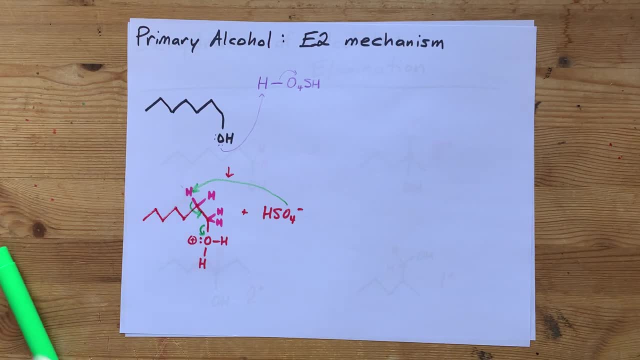 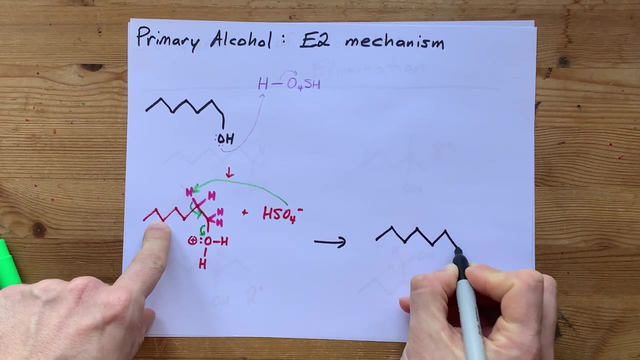 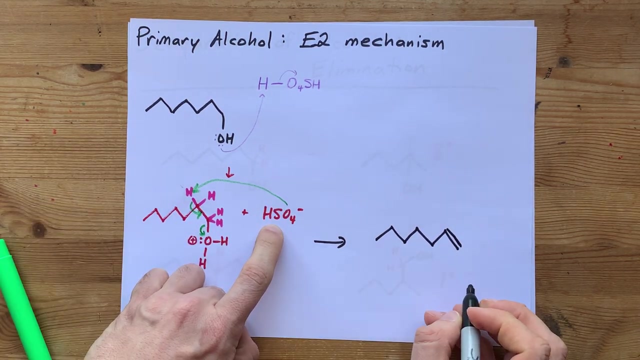 between the two carbons that are there. In the end, our product. here I still have the long carbon chain. Oh, am I missing one more? There we go. Except now I have a double bond. at the end The HSO4- took its extra H, so it's now H2SO4,. 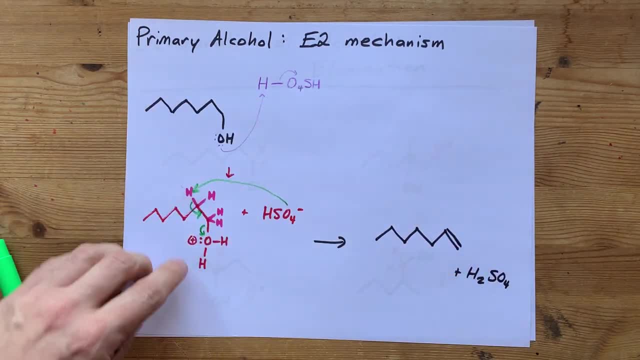 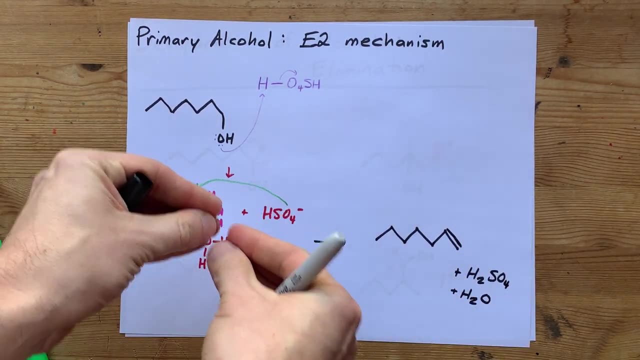 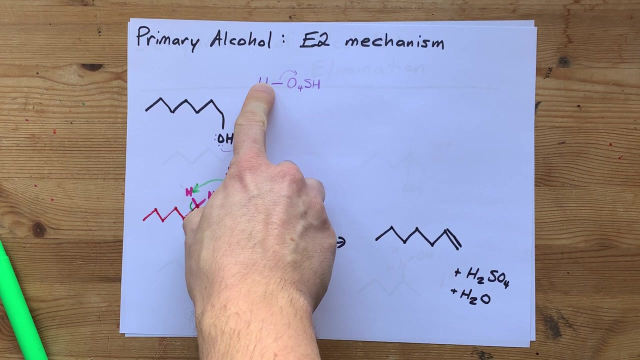 which is actually how it started. So it's a catalyst and you have H2O as a product. Ah, look dehydration, because you're taking a water out of the molecule total. Now, granted, this hydrogen came from the acid and the other the new hydrogen. that's. 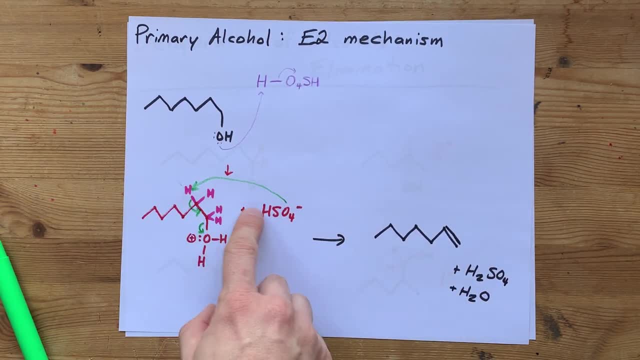 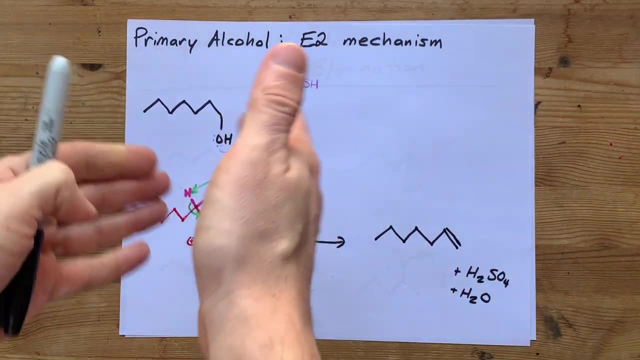 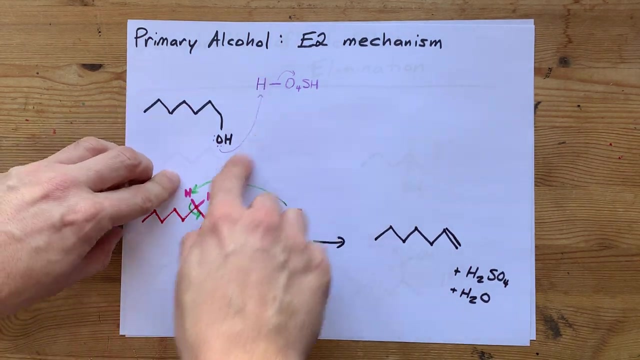 attached to this. HSO4 came from the carbon chain, but hydrogens are not like. you can't tell the difference between those unless you make one, some kind of weird isotope, and that's probably how we figured out what the mechanism was. but the point is that you're protonating the OH to 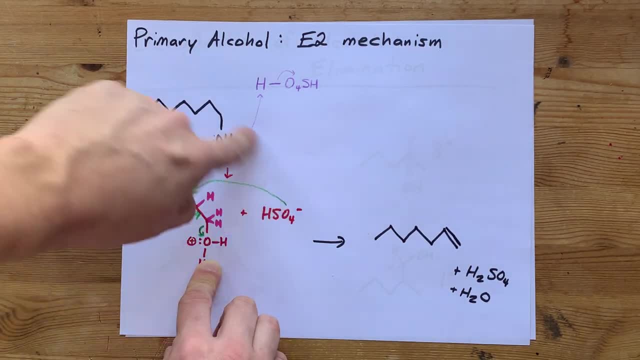 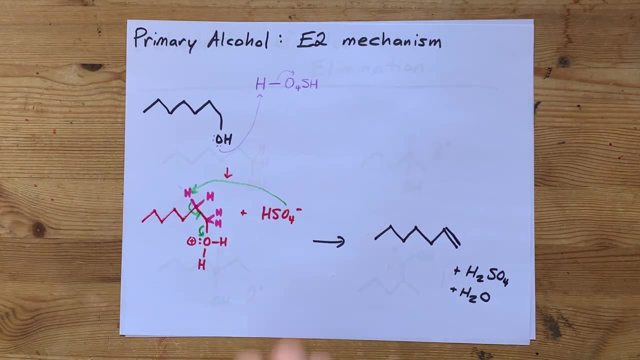 make it an OH2 group Super easy to leave. As long as you pluck a hydrogen off of the next carbon in the chain, the electrons flow around to create that double bond. It's beautiful. Please note that in what I believe is the rate determining step, which is this one to that one, you have two. 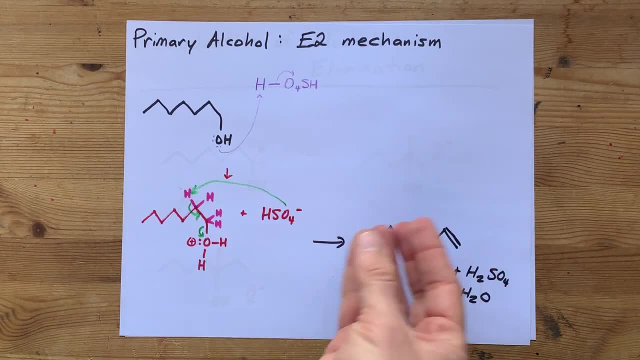 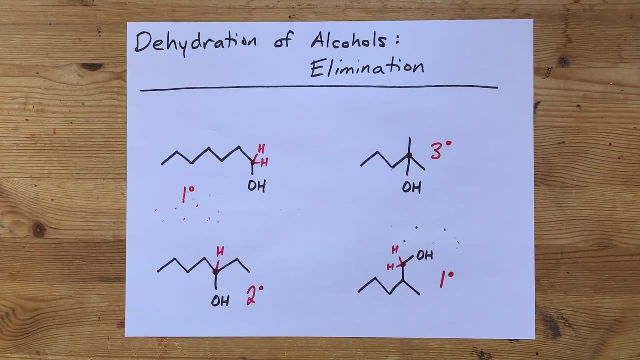 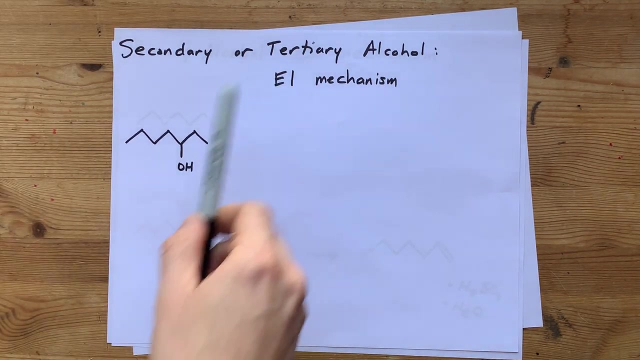 molecules colliding. That makes it a bimolecular reaction and that's why it's called E2.. Want to talk about E1?? I bet you. oh, that's not, that's not great. You want to talk about E1?? I bet you do. Let's go. So for E1, the one here represents. 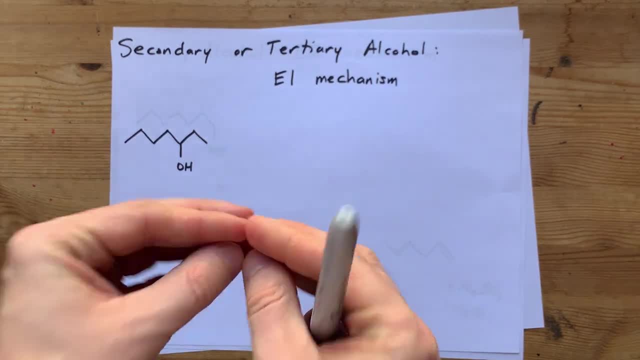 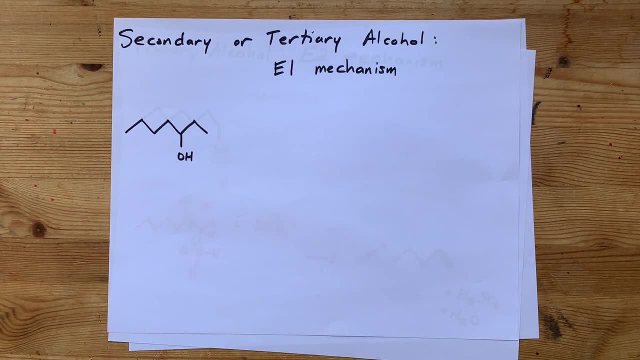 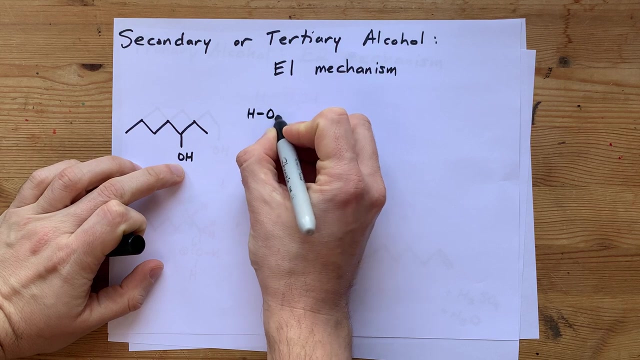 unimolecular. It is a single thing that is doing its magic in the rate limiting step. Okay, so what actually ends up happening here? We're still going to have to protonate the OH. I'm going to give you H2SO4 again. I don't know, I'm just picking an acid. 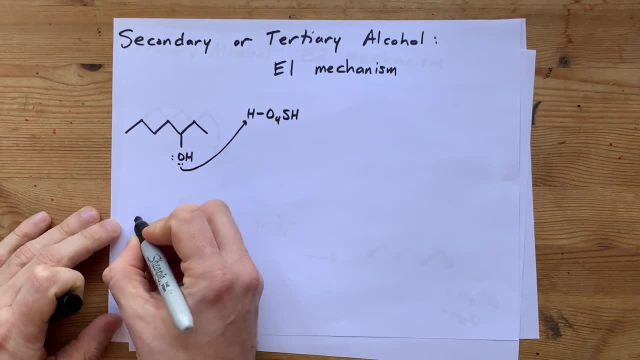 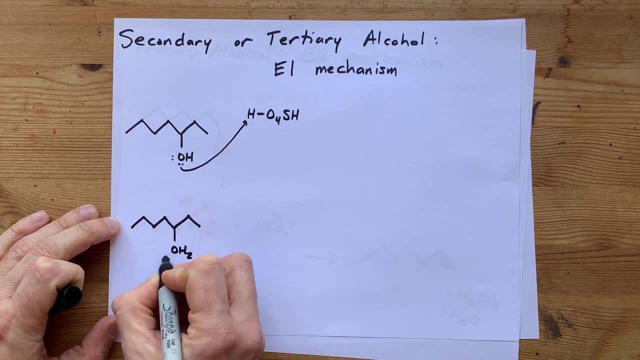 The lone pair. The lone pair on the water still steals the H. You still end up with the alko-oxonium ion. Here I've got OH2.. I'm just going to be a little. uh, there we go. We got our plus charge on the. 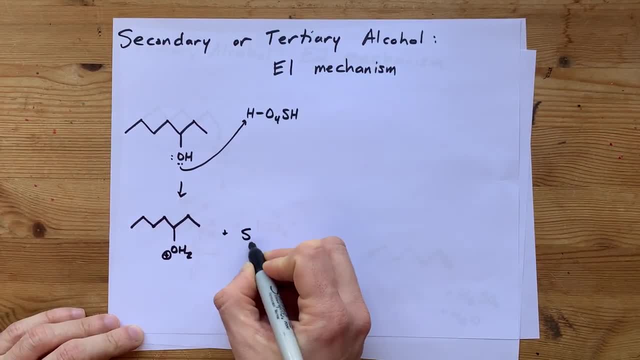 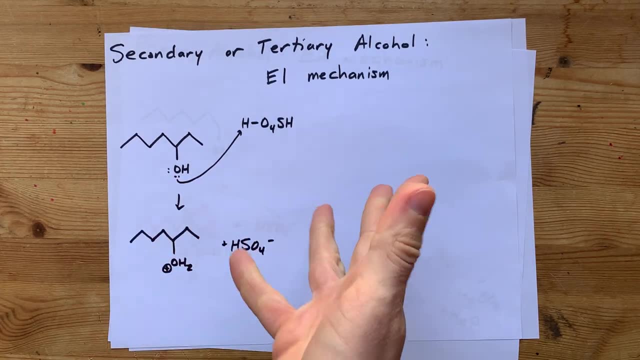 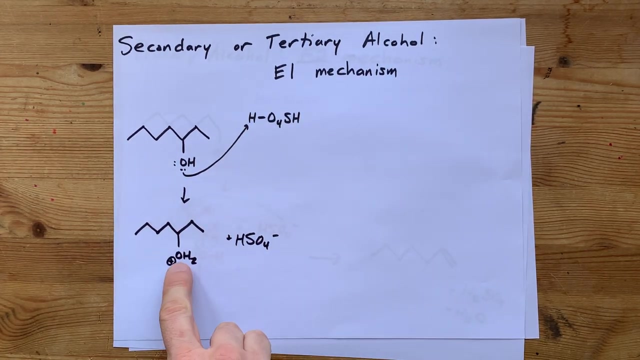 oxygen there And of course, we have the HSO4 minus that's left over. Okay, but that's easy. It's a strong acid. It gives away its H Piece of cake right Now for secondary or tertiary alcohols. what happens is that this OH2 is going to be a little bit more of a. you know. 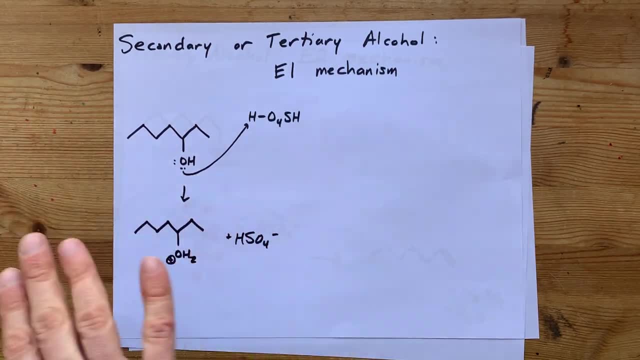 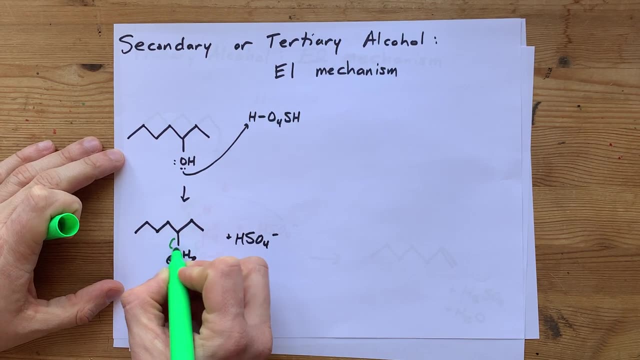 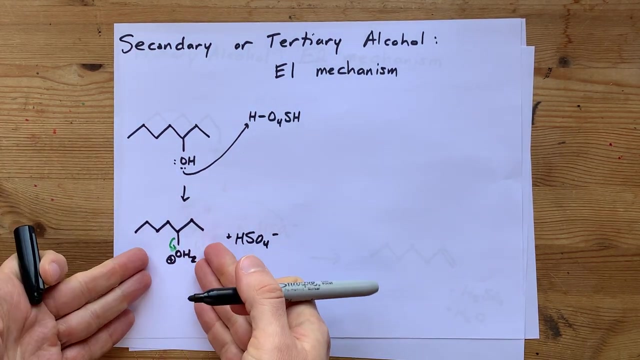 H2 actually falls off of the molecule entirely. The only electron flow happening here is going to be electrons flowing out of the covalent bond between carbon and oxygen straight to the water. This is a unimolecular decomposition because it's one molecule breaking apart into two. 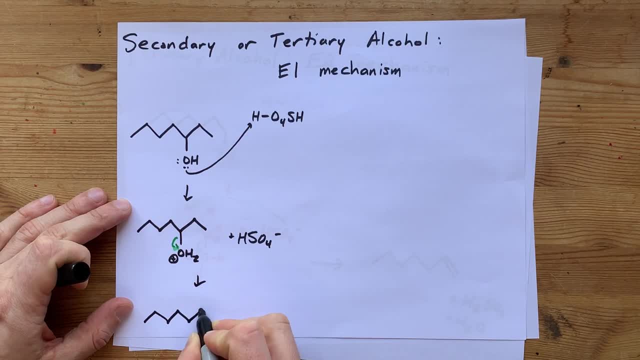 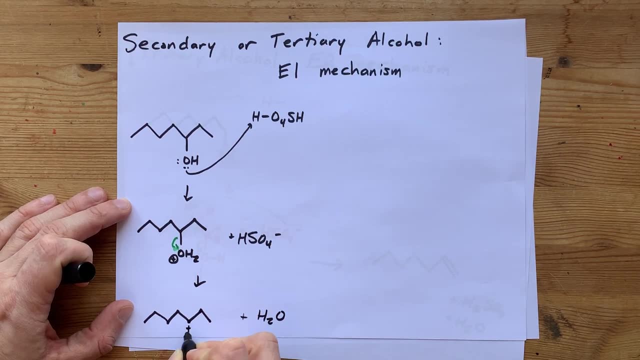 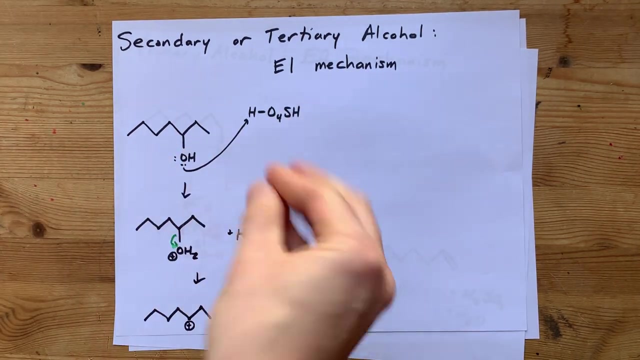 What you end up with is that same carbon chain, but now you've broken the water molecule off and you're left with a positive charge on this carbon, the carbon that the OH fell off of. This is why, or rather, this carbocation intermediate, is the reason this mechanism. 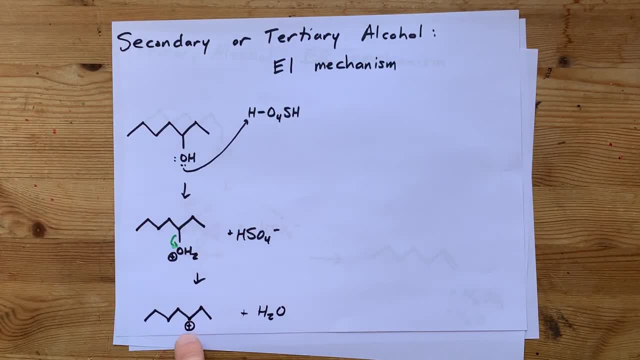 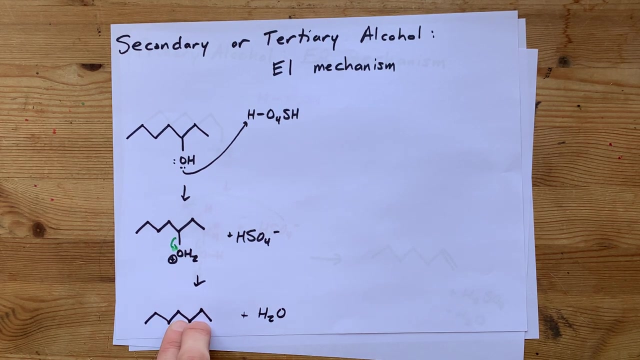 only occurs for secondary and tertiary alcohols. A primary carbocation, a plus charge on a carbon that isn't connected to more than two other carbons, is not very stable at all. You need that carbon that has the positive charge to be connected to at least two other carbons in order. 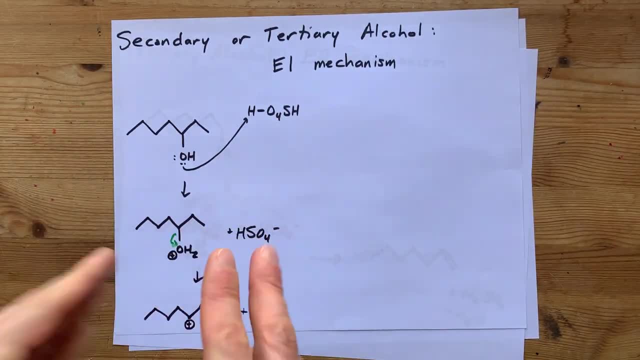 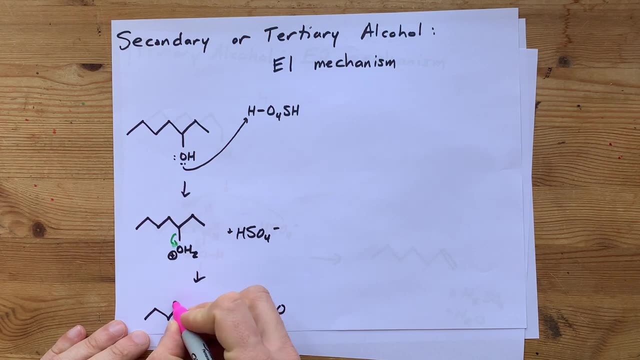 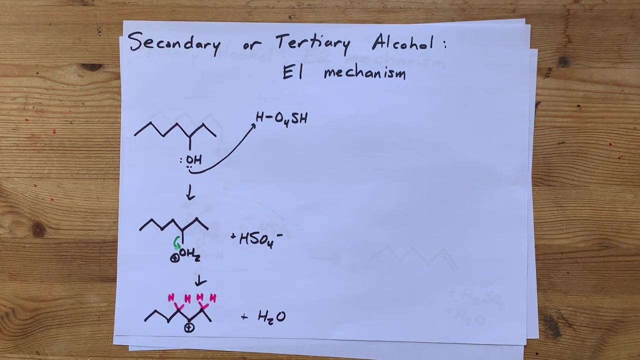 for it to be stable enough to operate as this intermediate. Great. Now I want to point out that you have two hydrogens connected to this carbon and two hydrogens connected to this carbon. Which hydrogen gets plucked off of the molecule will depend on a few different factors. 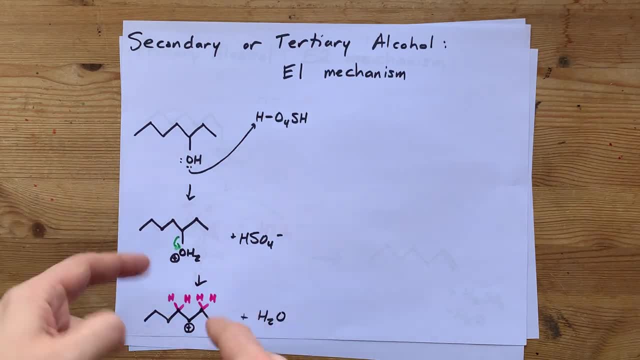 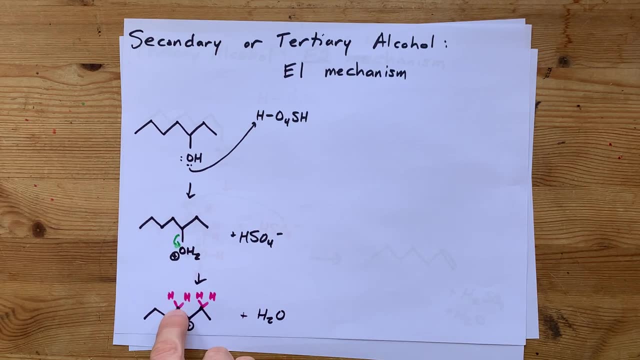 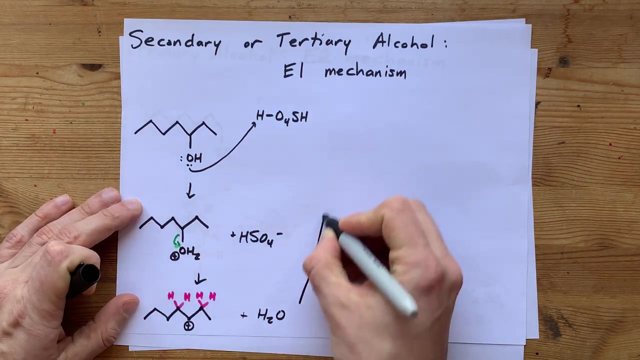 like if there's blocking groups or steric hindrance etc. etc. But for a molecule this simple, where it's just two H's over here and two H's over here, you can probably get away with grabbing either one. In fact, let's show that happening to both. Now the H2O, or maybe we'll. 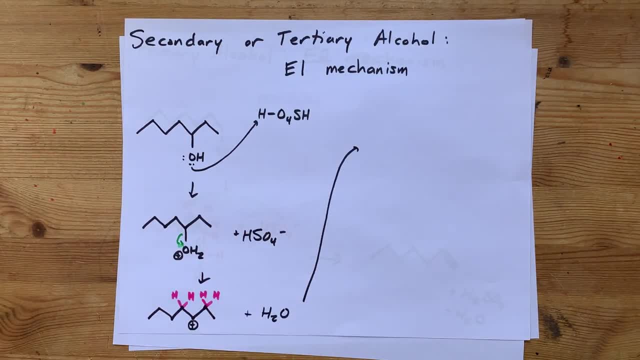 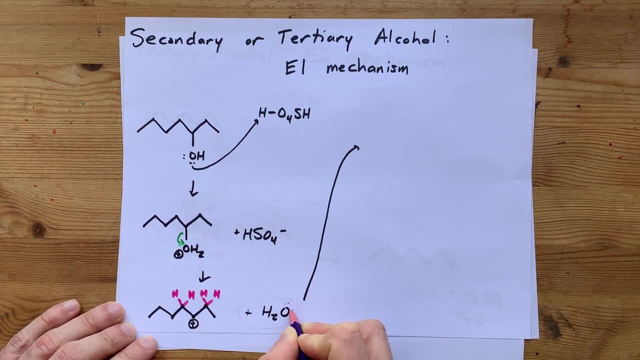 use the HSO4 here. something needs to steal this hydrogen away. I think I'm going to choose the water to make that happen. I'm going to choose the water to make that happen. I'm going to choose the water to make that happen. The water molecule is going to steal, let's say that, H away Where? 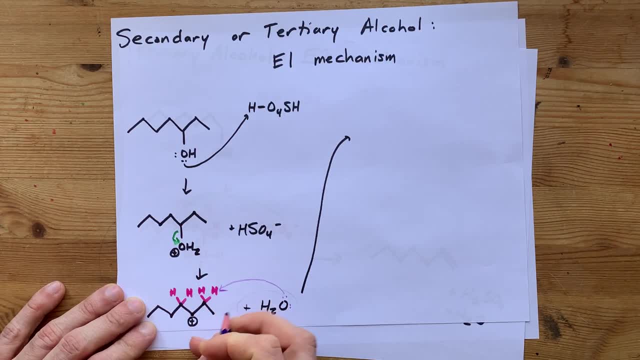 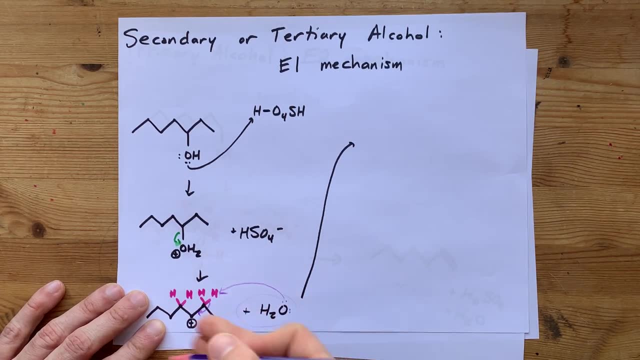 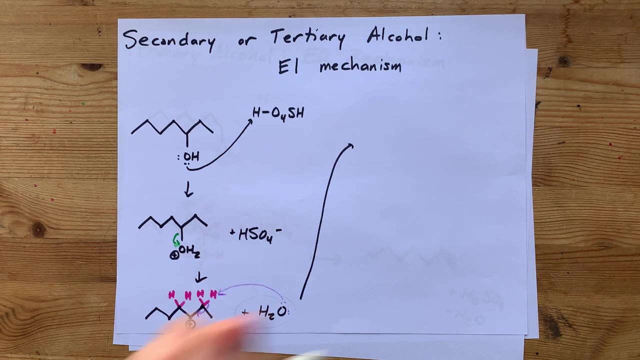 are the electrons from this covalent bond going to go? Well, they're going to flow towards the positive charge, because electrons are negatively charged and negatives and positives attract each other. right? If you pluck a hydrogen off of this carbon here, then your resulting molecule 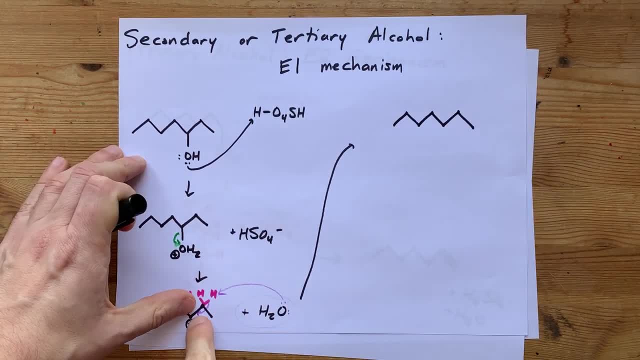 will have a negative charge. So if you pluck a hydrogen off of this carbon here, then your resulting molecule will have a negative charge, have a double bond between those two carbons. Now is it going to end up being cis or trans? 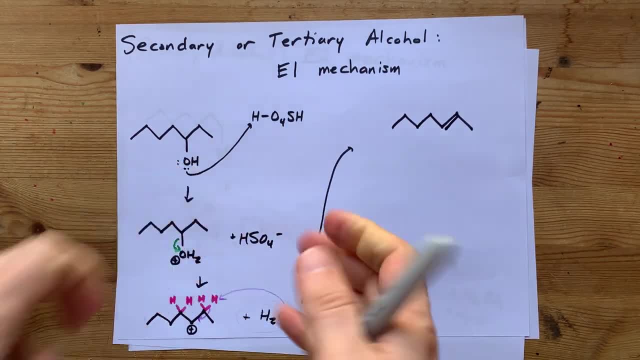 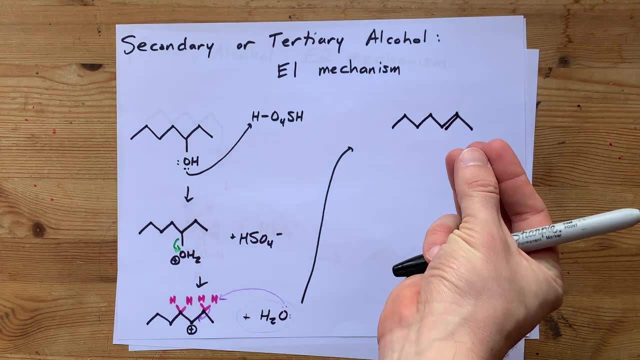 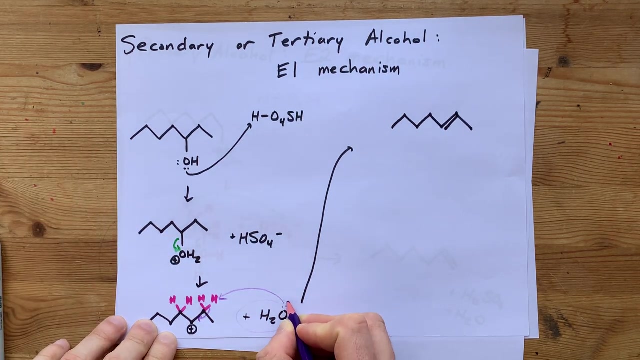 As far as I recall, trans is preferred as the product. It's not specific in that it's 100% trans, but trans is the major product as opposed to cis. okay, You could just as easily have had the water pluck off one of these hydrogens. in that case, You could just as easily have had the water. 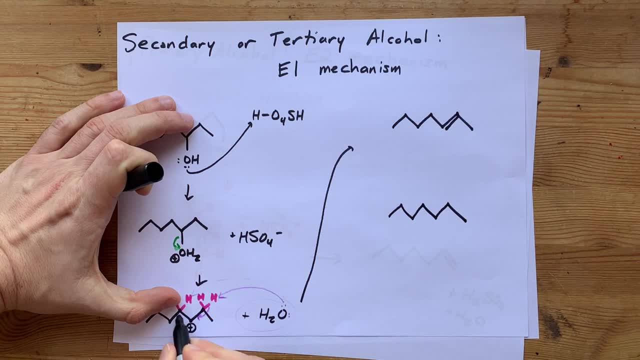 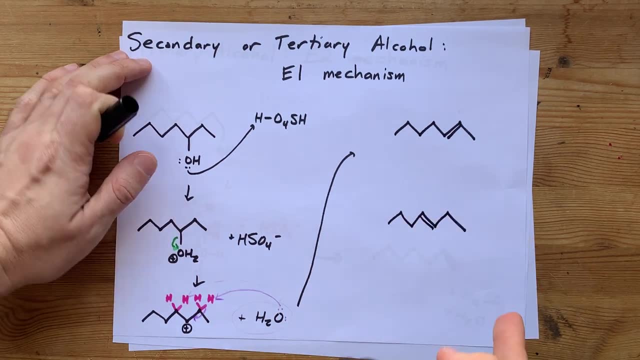 pluck off one of these hydrogens. in that case, You would have ended up with your double bond between these two carbons: the carbon that had the positive charge and the carbon you pluck the hydrogen off of. And again, I'm going to draw that as trans Now, because you have hydrogens on.